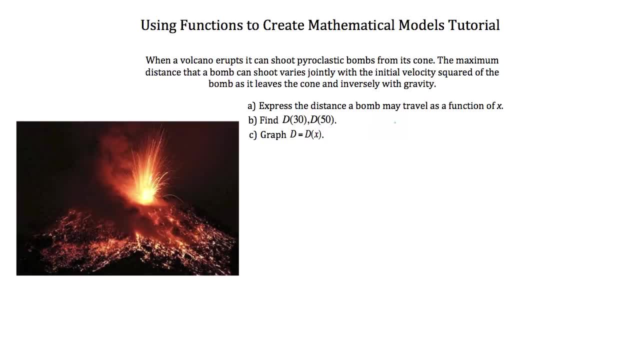 So question A is to express the distance a bomb may travel as a function of x. So we're going to write our function and we're calculating distance here. so I'm going to call our function d of x. Now we were told that a bomb can travel as a function of x. 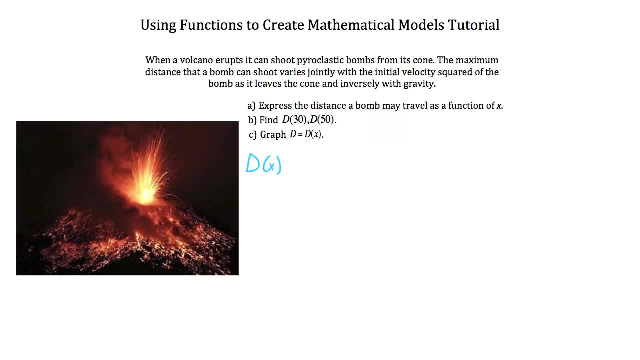 Now we're told that the maximum distance, the d that a bomb can shoot, is going to vary jointly with the initial velocity squared. So I'm going to make our initial velocity our x value, because it depends on what that velocity is And it's varying jointly here with our distance. so our velocity squared varies jointly with our distance. 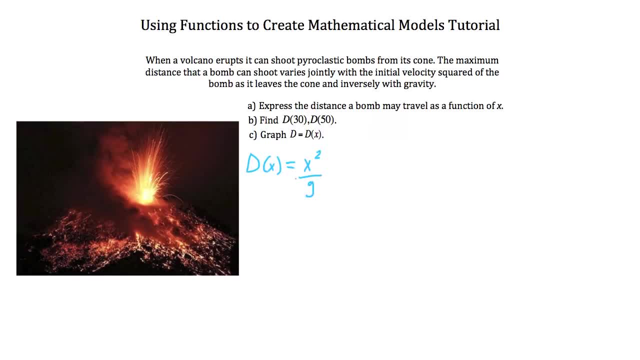 and inversely with gravity. And I'll just write g for gravity, And usually in physics they use 9.81 meters per second squared for gravity. And I'll just write g for gravity, And usually in physics they use 9.81 meters per second squared for gravity. 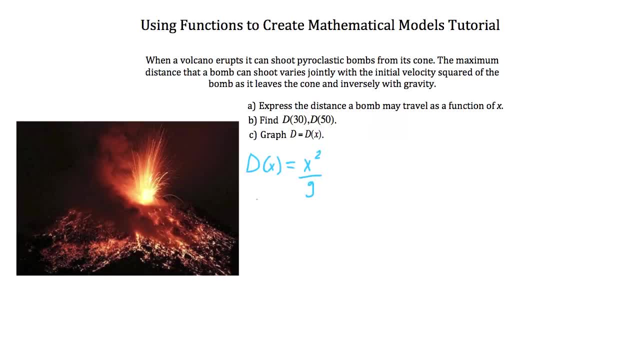 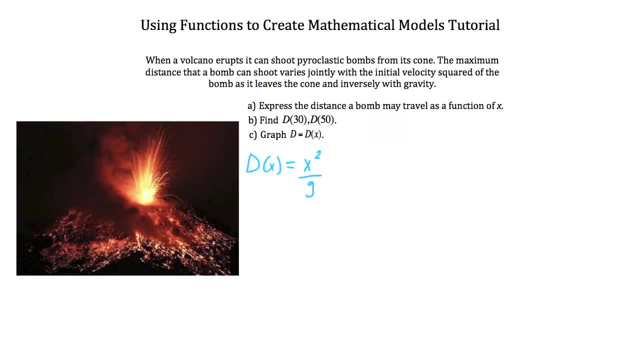 So d of 30 is equal to 30 squared divided by our gravity, which is 9.81 meters per second squared. So let's write our d of 30 down below here, d of 30, and we're going to plug in 30 for 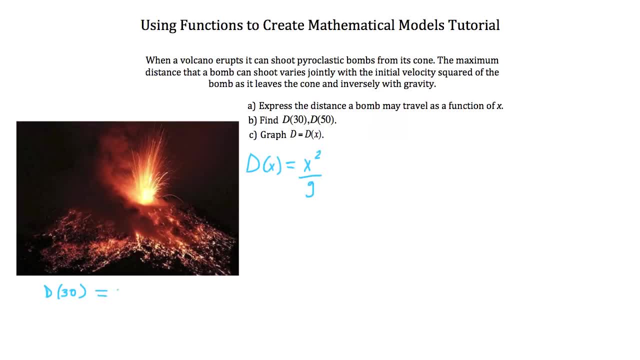 x. So d of 30 is equal to 30 squared divided by our gravity, which is 9.81 meters per second squared. So if we do that work, we find our d value, our distance, for this particular pyroclastic. 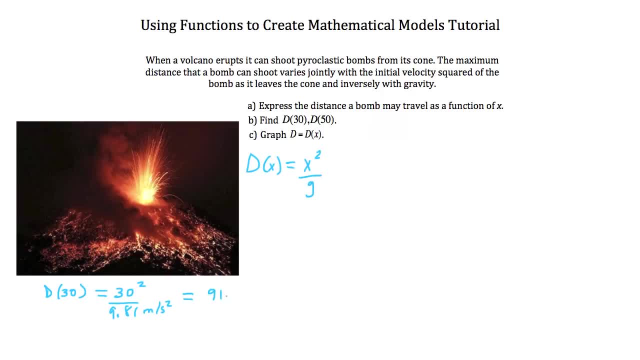 bomb is going to be 91.75 meters And a pyroclastic bomb are these pieces that are being ejected from the volcano, And you can get some really large ones. I mean from as small as a football to the size of a desk, being ejected from the cone of a volcano. 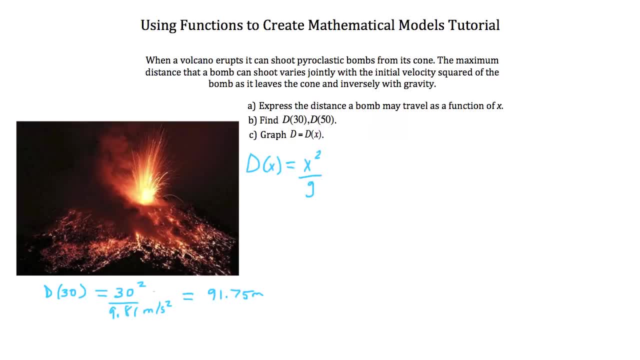 This particular pyroclastic bomb, if it were ejected at a velocity of 30 meters per second, is going to travel roughly the length of a football field, Which is pretty far. Now let's take a look at how far it would travel if it were going slightly faster. 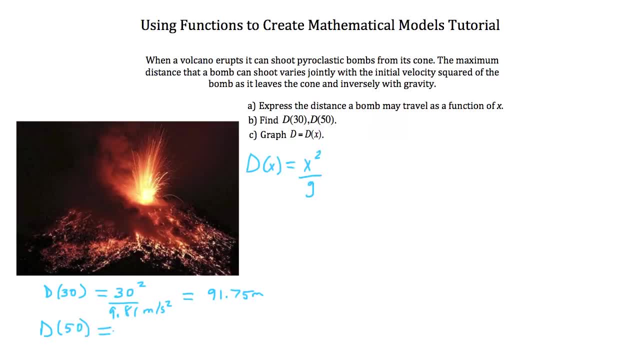 So if it were ejected at 50 meters per second? So we want to take our x value squared divided by gravity, which is 9.81, and that's meters per second squared, and our top value is meters per second And we get 254 meters per second. 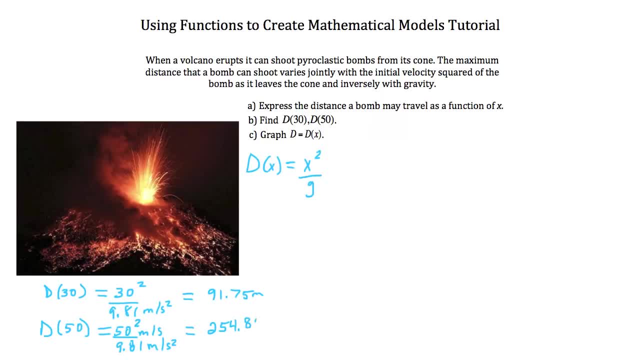 Okay, 0.84 meters. Notice how drastic this difference is. Our speed hasn't doubled, but our distance that that pyroclastic bomb has traveled, has doubled, More than So. that's one way we've used functions to create a mathematical model based on this. 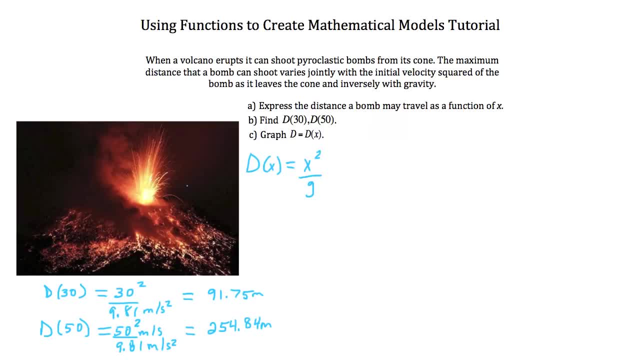 distance here of material being ejected from a volcano. This is actually a real formula that scientists use to study. Okay, Let's take a look at C. C asks us to graph this particular mathematical function. This is the graph that we're going to have for this function, and if you plug our function, 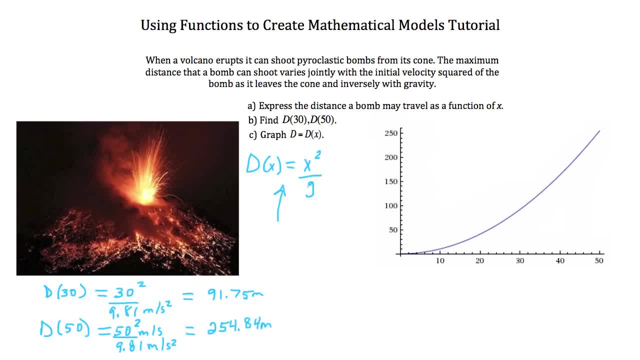 directly into your calculator and use 9.81 for your g. you're going to get this graph And you'll notice you can use it also to find those values for b On our x coordinate. here down on the bottom you're going to have that initial velocity and our y coordinate. 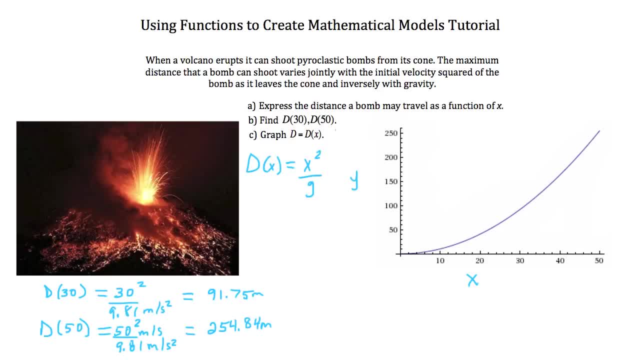 over here is going to give you the total distance that that pyroclastic bomb traveled. So if you just drew a line directly up from 30, you'll see that it's just below 100.. And if you drew a line directly up from 50 here, you're going to see that it's just above. 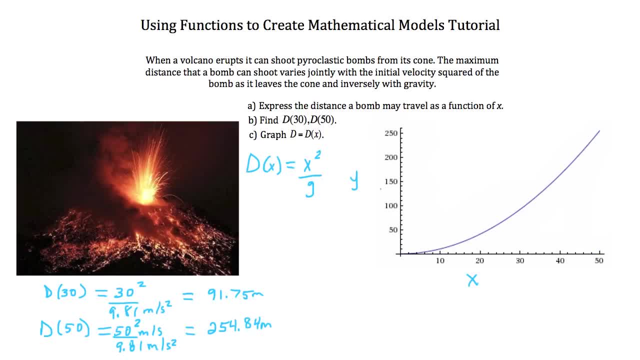 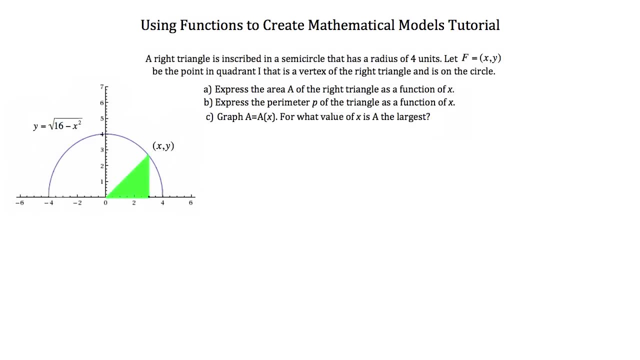 250 on the y axis. So sometimes that nice graph can really assist you And verifying a function and also simplifying your mathematical model. Now let's take a look at another math model. A right triangle is inscribed in a semicircle that has a radius of four units. 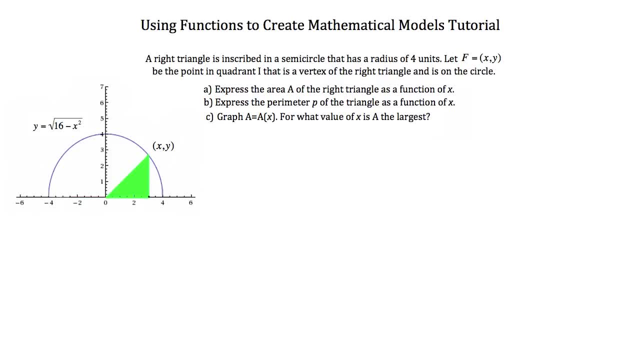 Let f equal x comma y, be the point in quadrant one that's a vertex of the right triangle and is on the circle. So here's our description, our drawing over here on the left. Notice that this is the point f, here that x comma y coordinate right there on the edge. 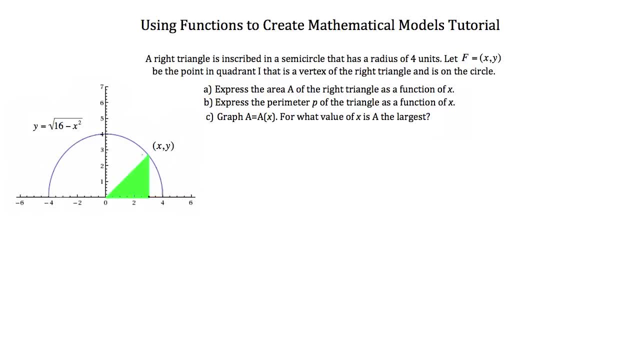 of our circle And it's inside quadrant one of our graph. So a asks us to express the area a of the right triangle as a function of x. Now remember, the area of a right triangle is equal to one half the base times the height. 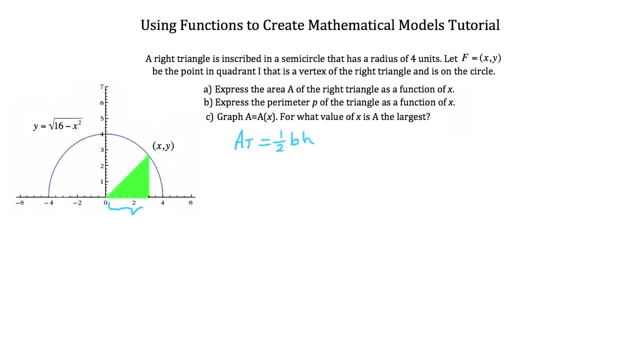 Now we could consider the base of our triangle to be here Along the x axis, And it's going to be whatever that x coordinate is. We don't know what it is, but that would be our base, And the height of our right triangle is right here. 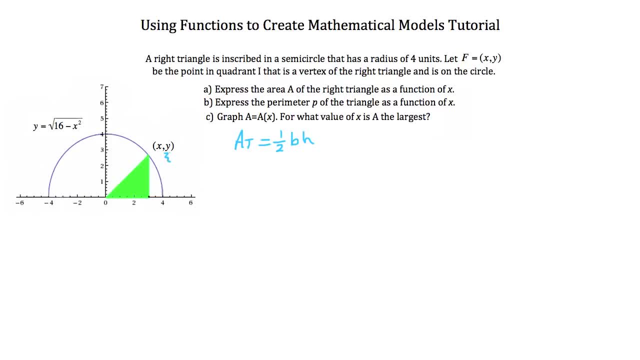 And that's going to be our y coordinate, That's going to be the total height. For example, if you just eyeballed it and you said: okay, the graph looks like it's about two and a half units high on our graph, then our y coordinate would be 2.5.. 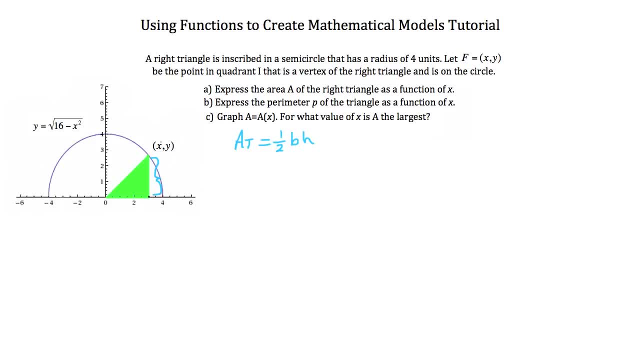 And that would actually be the height of this triangle as well, Nix, So a way that we can write that is a the area of the right triangle and x here. so our function a of x is going to be equal to one half of our x times our y. 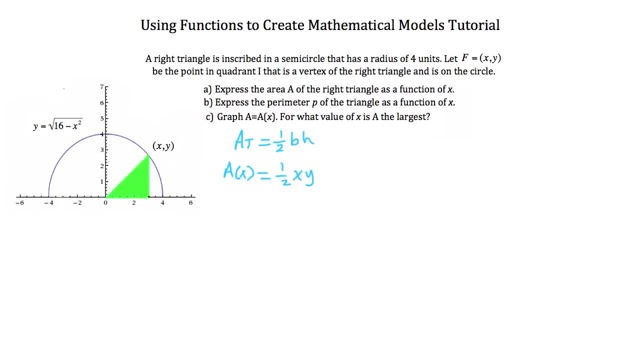 And notice that the y value here is our y value from the function that created this circle. Okay, The circle is over here. y is equal to the square root of 16 minus x squared, So let's plug that in for our y value here in our function. 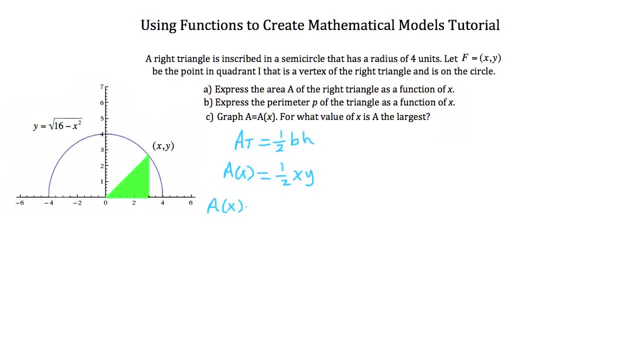 So a of x is equal to 1 half of x times that y value, which is the square root of 16 minus x squared. So this is going to be the function that represents the area of our right triangle. Now let's take a look at part b here. 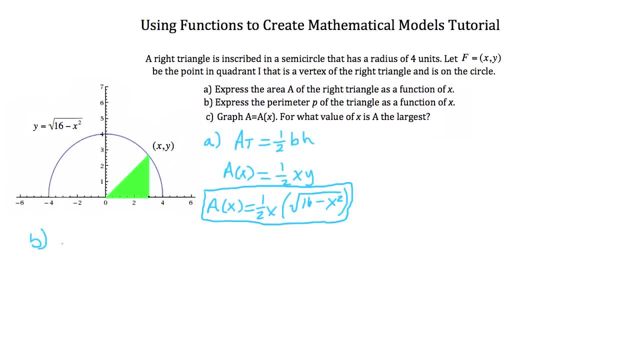 Part b asks us to express the perimeter p of the triangle as a function of x. So the perimeter of a triangle is the sum of the lengths of all three sides, and we know that this side has a length of x, this side has a length of y, and this side we can use. 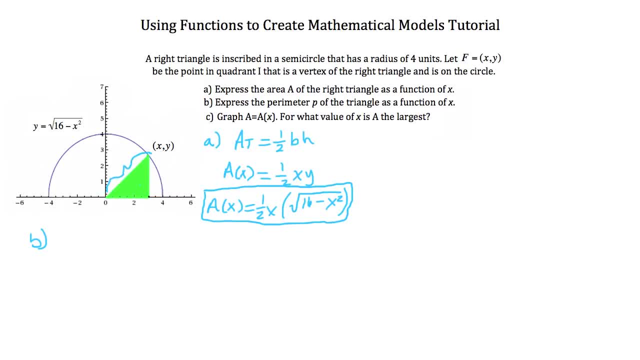 the distance formula to calculate. So the perimeter for our right triangle is p, is equal to x plus y plus the distance, and this is where the distance formula comes into effect: x minus 0 squared plus y minus 0 squared. Now the reason I use 0 and 0 here is the distance formula is x2 minus x1.. 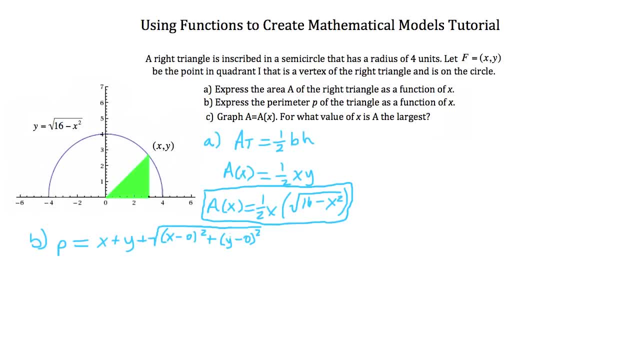 So I have y1 squared plus y2 minus y1 squared And I used our x1, y1 point to be right here at the origin 0, 0.. So that's where the x1 and y1 got their zeros. 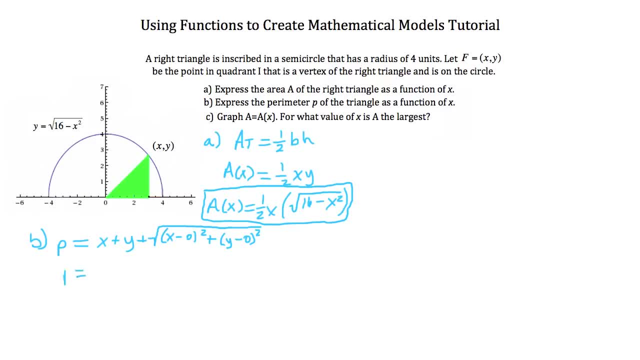 So we can factor that down or simplify here: p is equal to x plus y, plus the square root of x squared plus y squared. So now let's go ahead and plug in our y formula here And do the y's in our function. 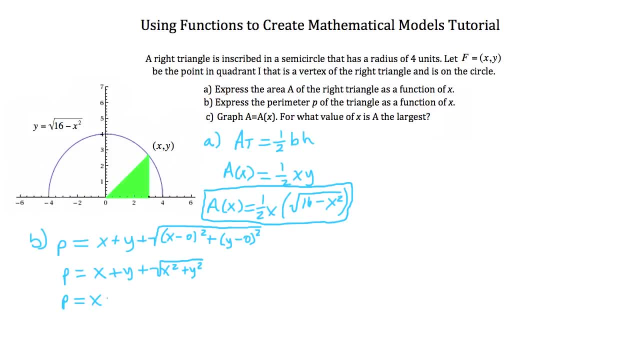 So p is equal to x plus the root of 16 minus x squared plus the square root of x squared plus y, which is the square root of 16 minus x squared squared, Now the square root of 16 minus x squared all squared. 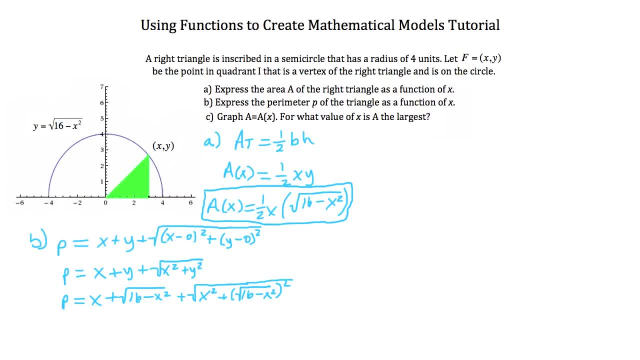 So we've got: p is equal to x plus the root of 16 minus x squared, plus the square root of x squared plus 16 minus x squared. So our x squared and our minus x squared are going to cancel each other out and we're left. 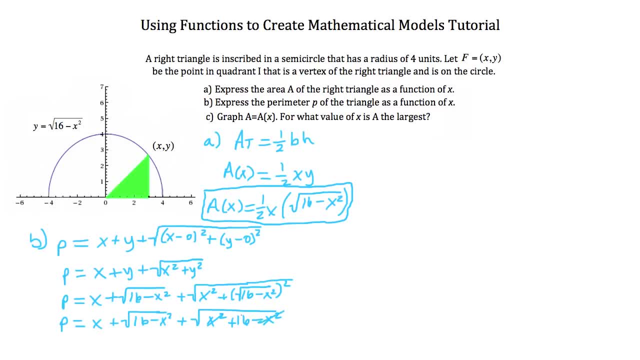 with the root of 16, which is 4.. So what we have here is p is equal to x plus 4 plus the square root of 16 minus x squared. So now we've created a function of the perimeter of our right triangle as a function of x. 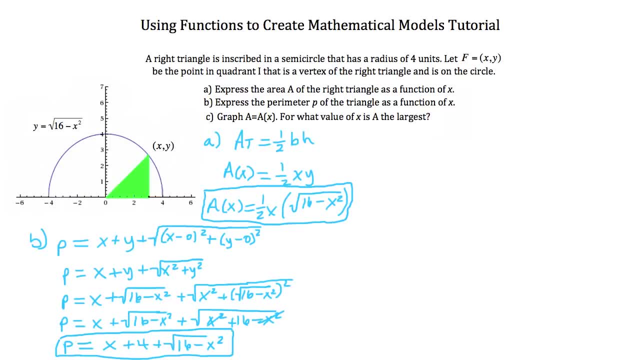 So, lastly, we've been asked to graph a of a of x. for what value of x is a the largest? So I'm going to start with a. Let's start with graphing that, And to graph it. you just want to put this function into your calculator. 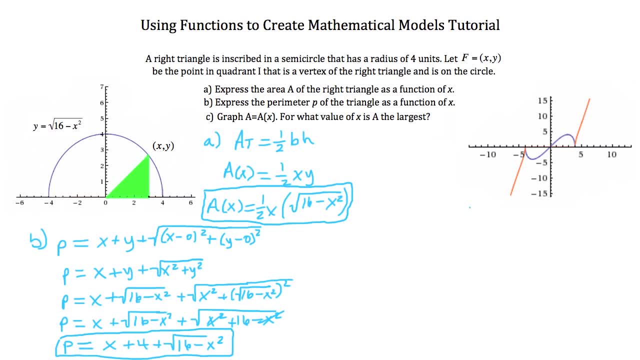 When you do, it's going to look like this. Now, the orange lines- there are all the irrational values for this function, so you don't have to worry about those. What you're really concerned about is those blue lines. That's the actual graph of your function. 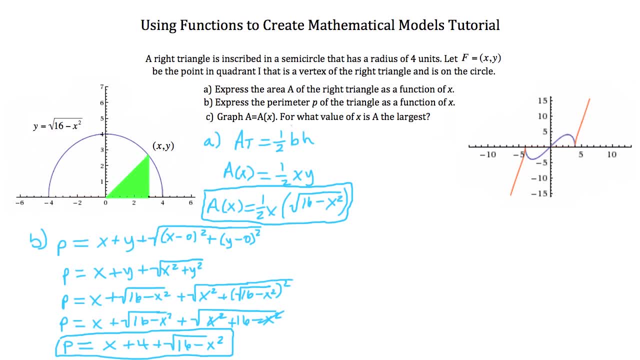 Now the second part to the question is: for what value of x is a the largest? Well, a is the area of your right triangle And since that's what you put in for your graph here, essentially whatever value of x looks like it's going to be the largest, here is going to return you the largest area. 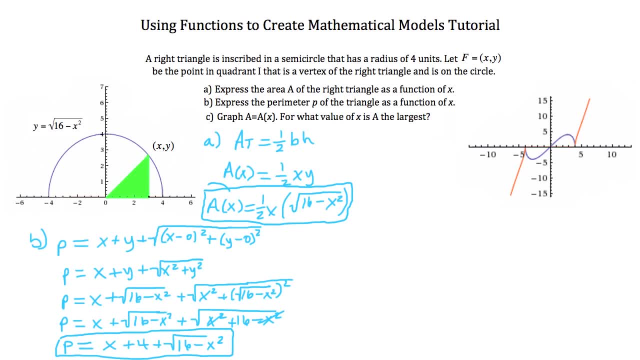 Because y now has been made from our a of x, so the highest y value is the highest a of x value. a of x is our area, So you want to look at what x value gets you to the highest point on our graph And one way of doing that, the most accurate way of doing that, with your 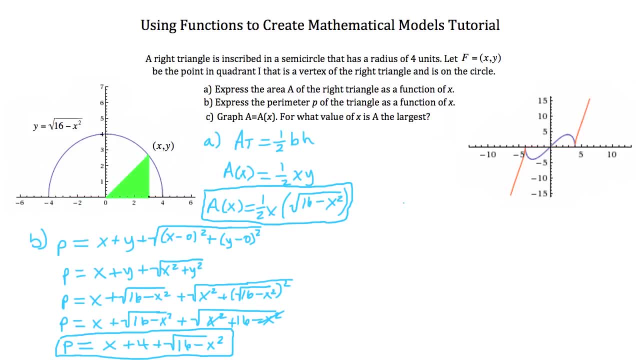 calculator is to use the maximum calculation on your calculator to calculate the maximum of this graph. When you do that, you find that x is equal to roughly 2.82.. That would give you an area of 4 if that were your x value 2.82.. Now for where you're at right now in 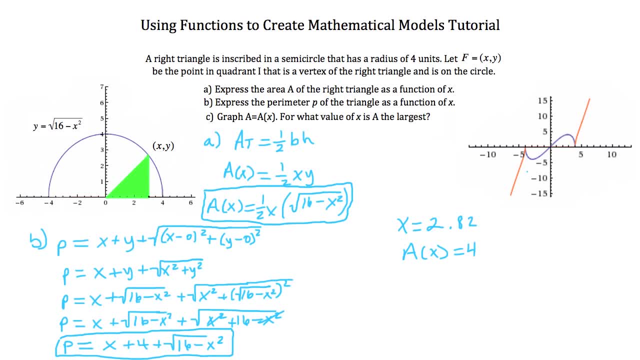 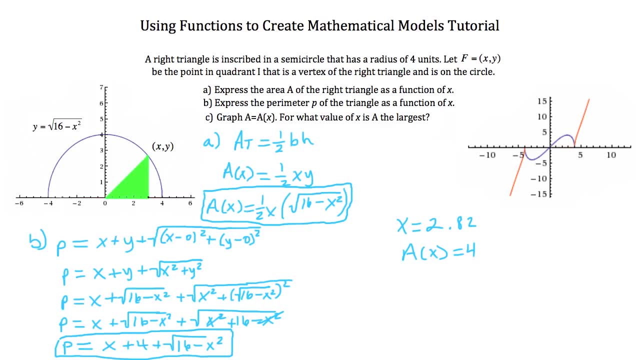 your knowledge of calculus, you want to either use your graph there to calculate it or use the maximum function on your calculator to find the area, Alright. so this is how we use functions to create mathematical models. Now, like I said at the beginning of this tutorial, 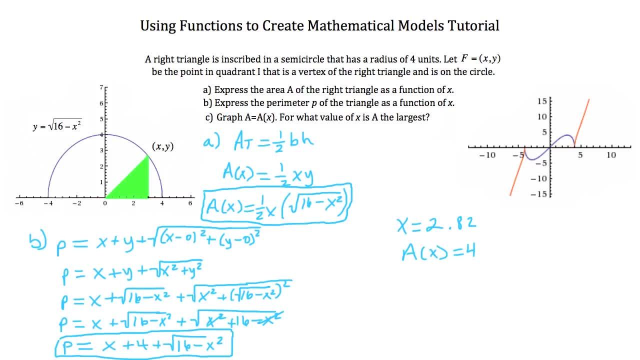 the functions that you've been learning in this tutorial can be pretty diverse, And that means that the mathematical models that you create can also be pretty diverse. So what that means for you is that you need to do a lot of these practice problems in this chapter in your work so that you can get used to the